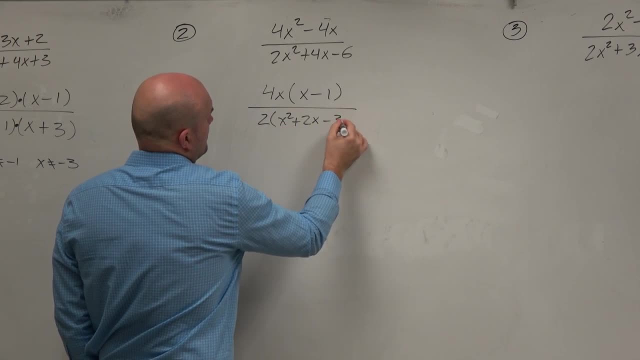 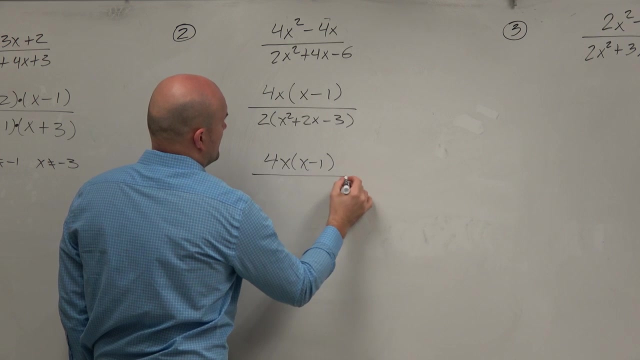 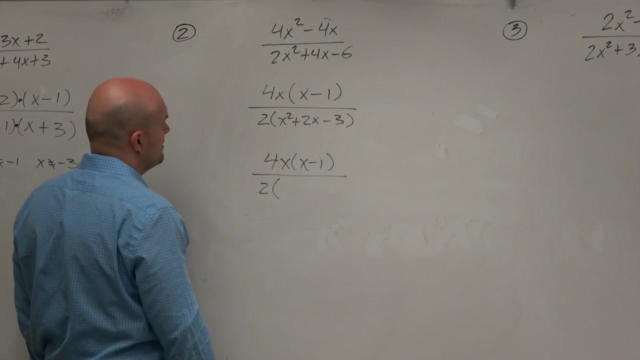 And I say: all right, well, I can factor that a little bit further down. So 4x times x minus 1, all over 2 times. let's see what two numbers multiply to give me, negative, 3 add to give me. did I mess that up again? I did. 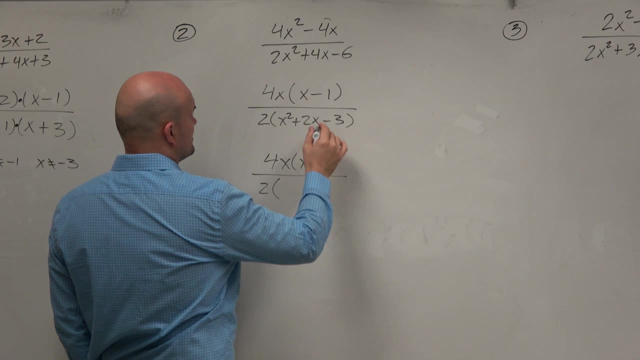 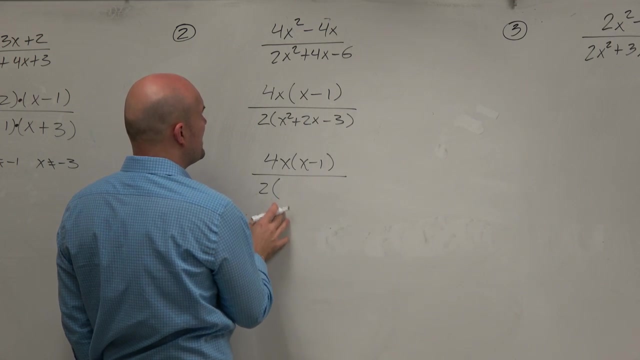 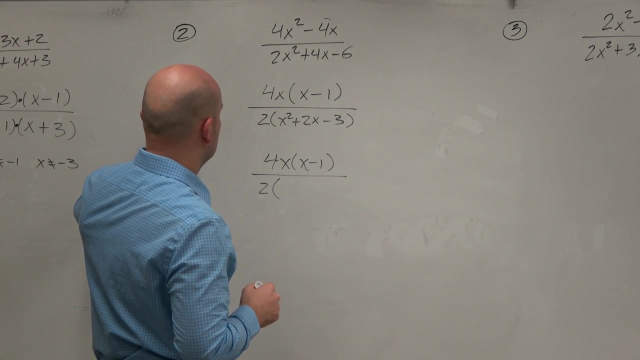 That was supposed to be a positive. Wait, no, that's an x minus 1.. Wait, that works right: x minus 3.. No, it's supposed to be a minus 1.. Hold on a second. Yeah, because it's x plus 3 times x minus 1.. 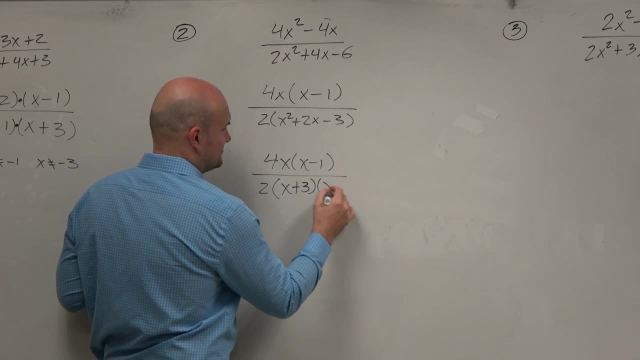 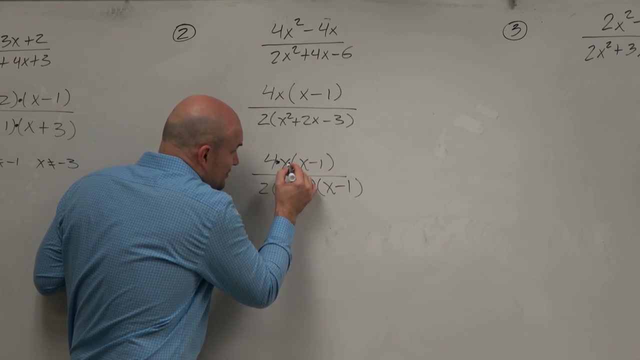 Yeah, it was OK. yeah, sorry, I'm right, I did write it. Thank you, I was, like I wrote it down in my paper, wrong in either case, All right. so now, in this case, by factoring, we have rewritten everything as a product of our factors. You guys see that. 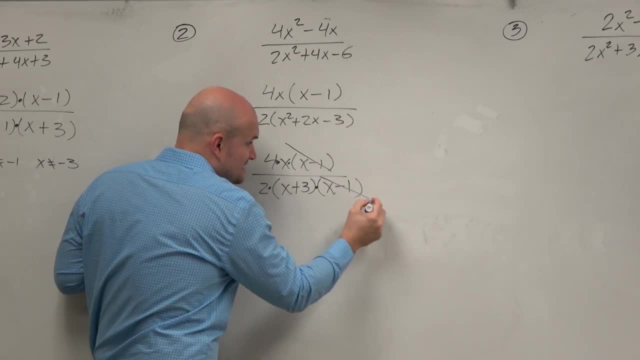 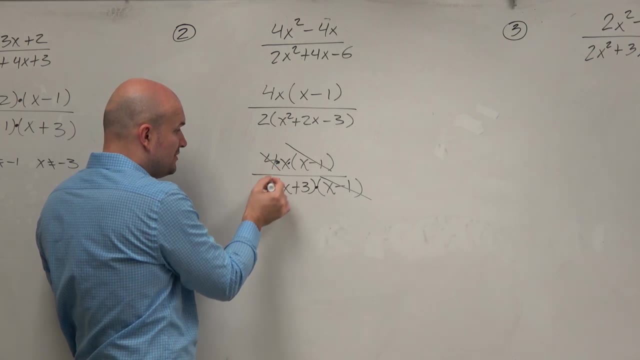 So now, Now I can apply the division property. These are just going to divide to 1.. 4 doesn't divide, and 4 divided by 2 doesn't divide to 1, but 4 over 2 can be reduced to 2 over 1.. 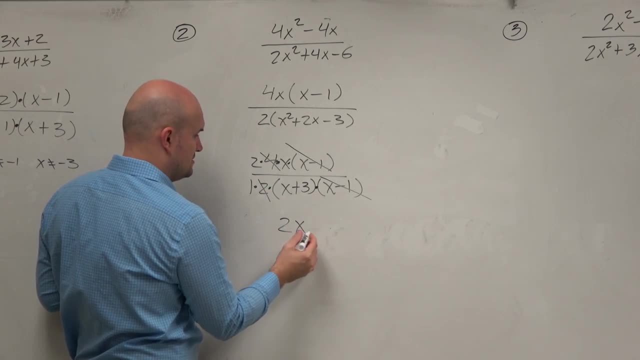 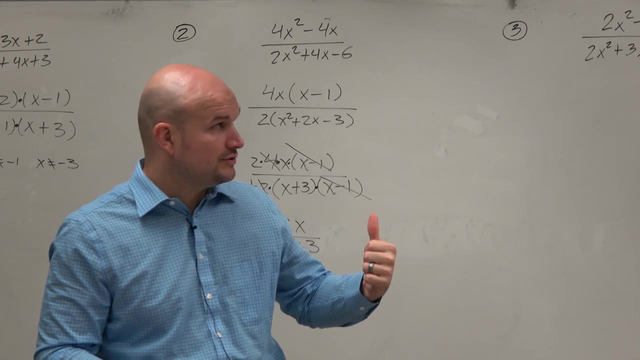 Right. So now what I have left is 2x and then denominator x plus 3.. OK, now it's important for us to go back when we're doing our restrictions. Don't do the restrictions just from here. Yes, x. 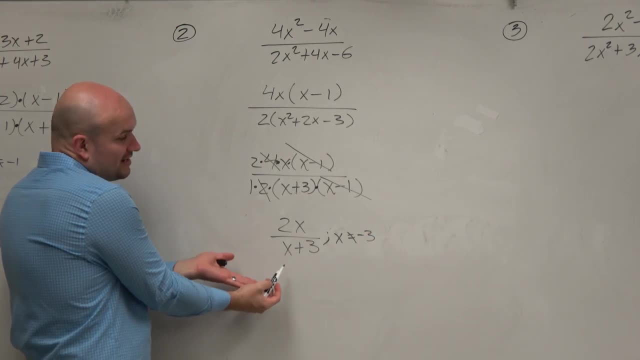 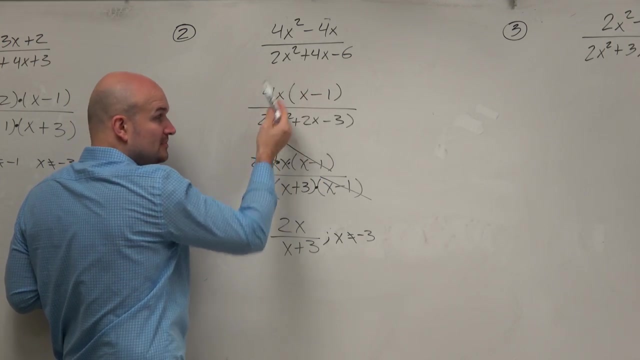 x cannot equal negative 3.. However, we're not going to define the restrictions from this simplified result. We need to take the restrictions from our original result as well. So I don't want to look at the restrictions here, not here. I want to look at them here before I simplified anything out. 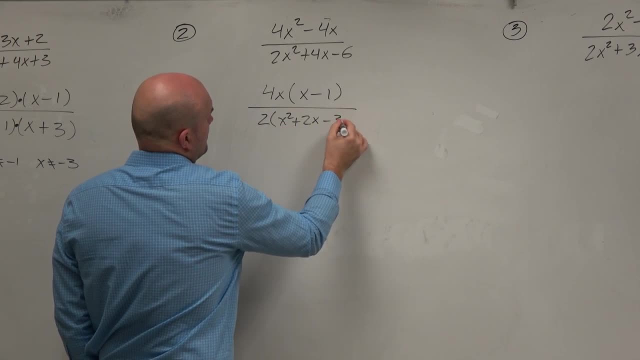 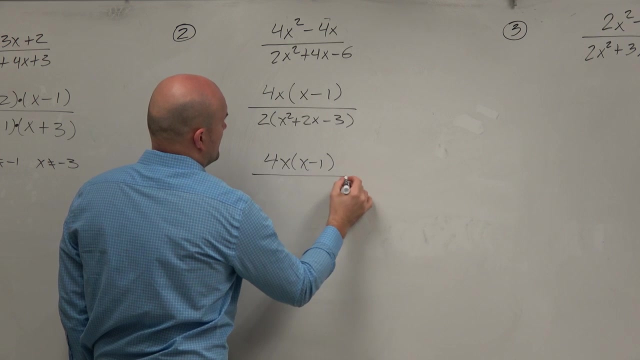 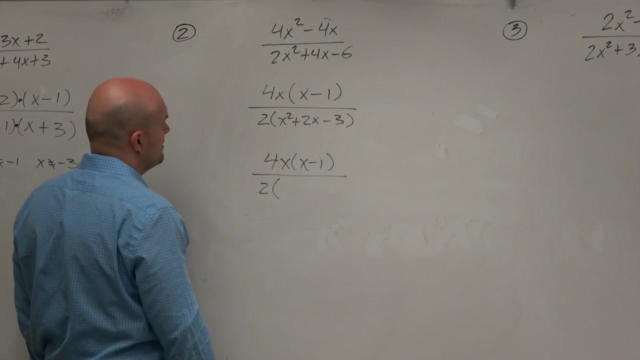 And I say: all right, well, I can factor that a little bit further down. So 4x times x minus 1, all over 2 times. let's see what two numbers multiply to give me, negative, 3 add to give me. did I mess that up again? I did. 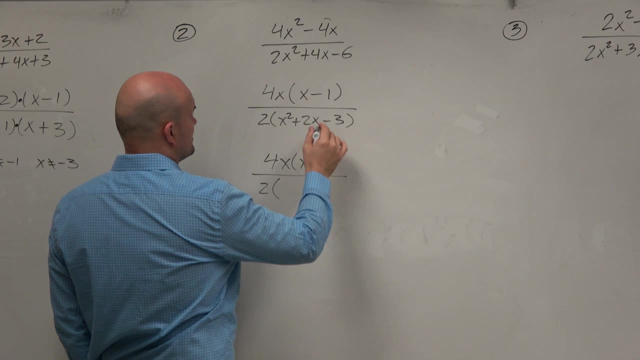 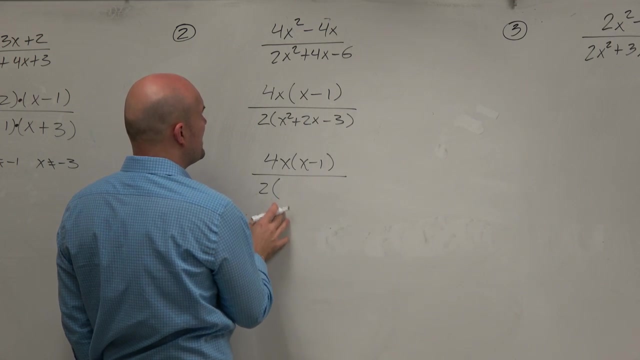 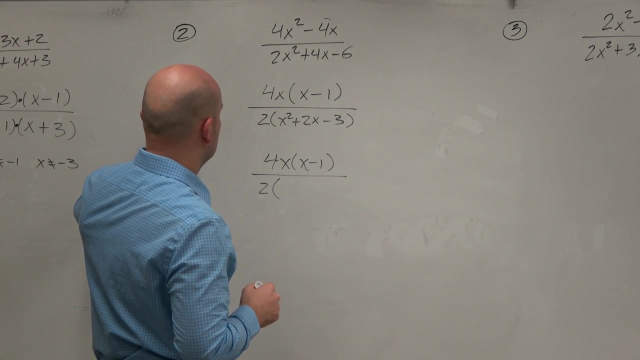 That was supposed to be a positive. Wait, no, that's an x minus 1.. Wait, that works right: x minus 3.. No, it's supposed to be a minus 1.. Hold on a second. Yeah, because it's x plus 3 times x minus 1.. 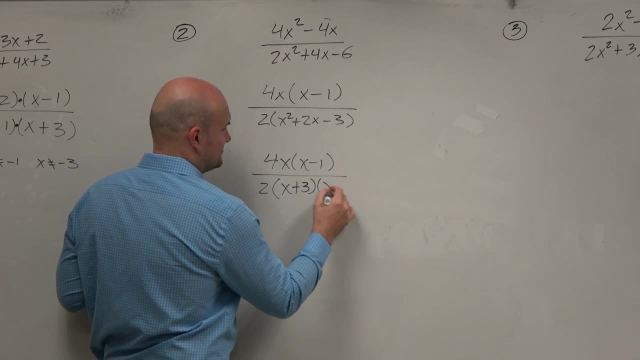 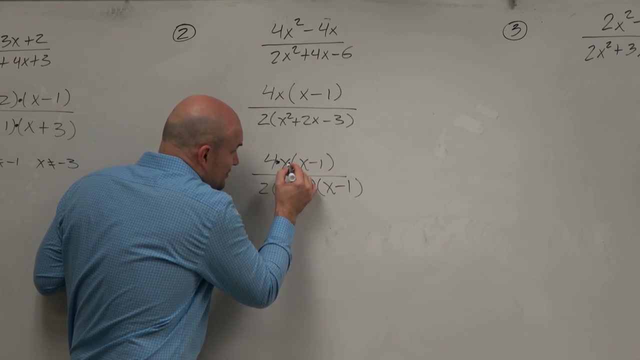 Yeah, it was OK. yeah, sorry, I'm right, I did write it. Thank you, I was, like I wrote it down in my paper, wrong in either case, All right. so now, in this case, by factoring, we have rewritten everything as a product of our factors. You guys see that. 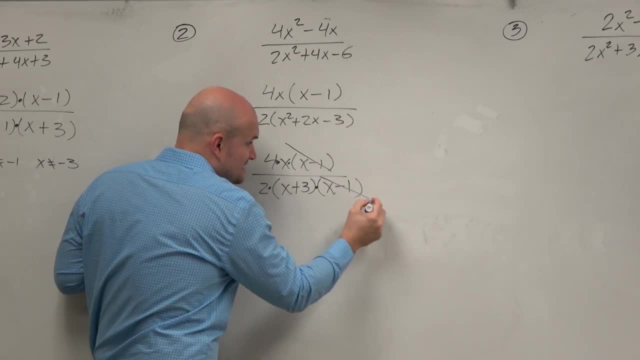 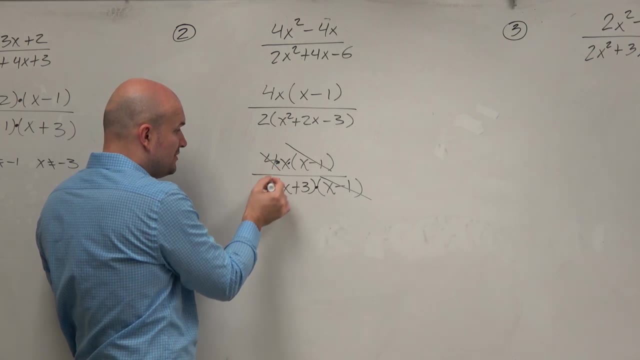 So now, Now I can apply the division property. These are just going to divide to 1.. 4 doesn't divide, and 4 divided by 2 doesn't divide to 1, but 4 over 2 can be reduced to 2 over 1.. 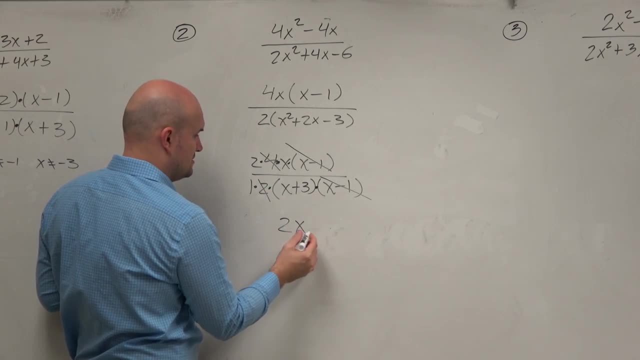 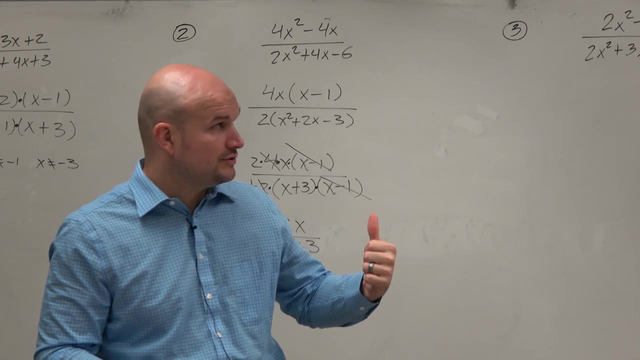 Right. So now what I have left is 2x and then denominator x plus 3.. OK, now it's important for us to go back when we're doing our restrictions. Don't do the restrictions just from here. Yes, x. 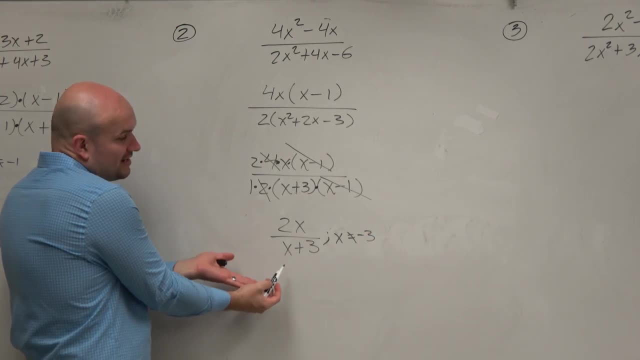 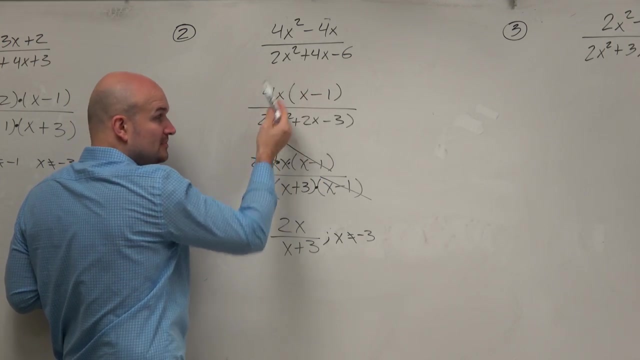 x cannot equal negative 3.. However, we're not going to define the restrictions from this simplified result. We need to take the restrictions from our original result as well. So I don't want to look at the restrictions here, not here. I want to look at them here before I simplified anything out. 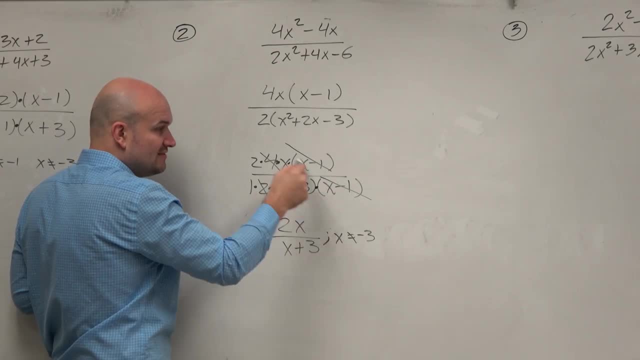 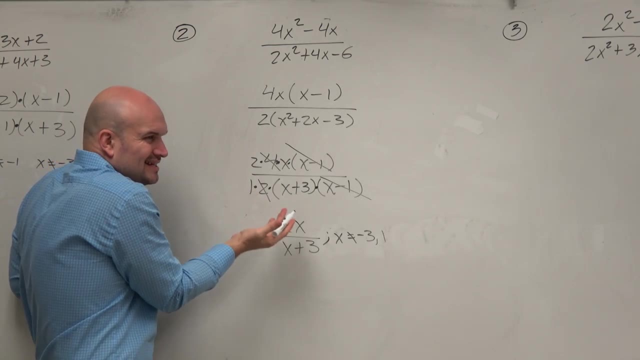 And was there any other numbers that x could not equal before I started dividing those out? 1.. What about 2?? No, 2's not a variable. It doesn't make that 0, right, So that doesn't make sense. 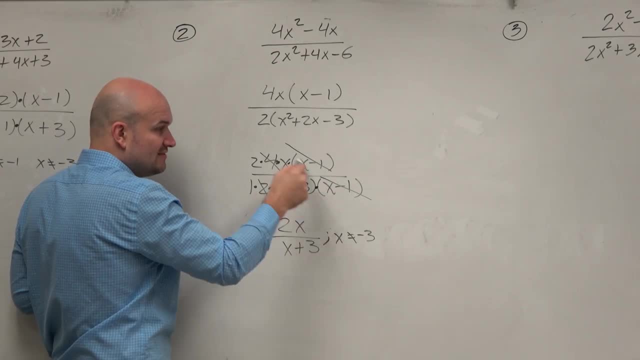 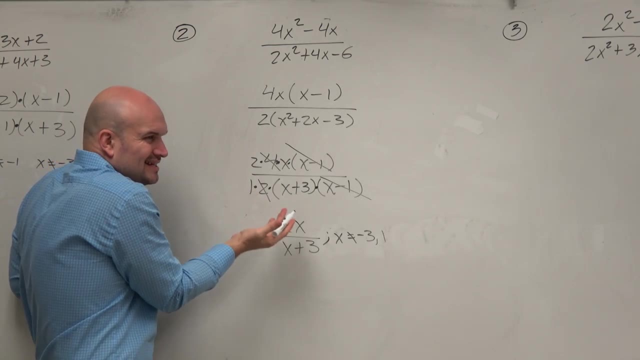 And was there any other numbers that x could not equal before I started dividing those out? 1.. What about 2?? No, 2's not a variable. It doesn't make that 0, right, So that doesn't make sense. 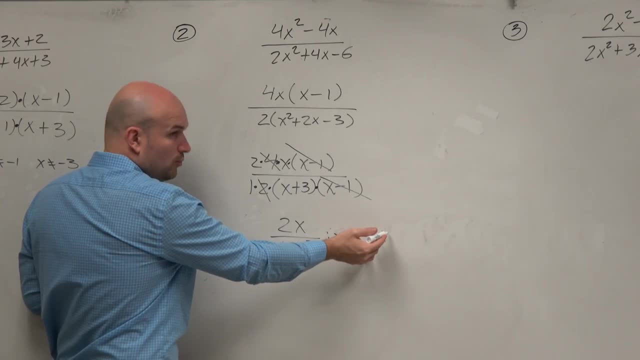 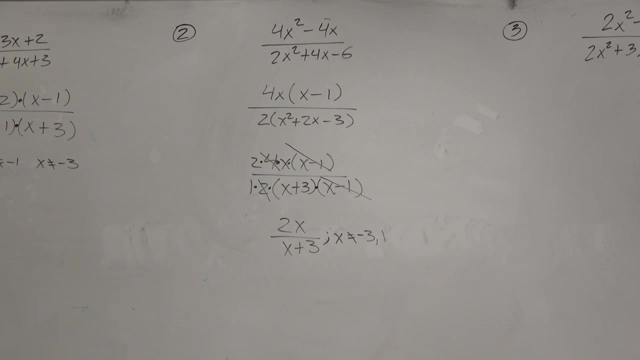 So my 2 undefined values, My 2 undefined values are: x cannot equal negative 3 or 1, because those would have made that 0. And again, you know it gets to the confusing part of, but it got divided out. Why is it still, you know, not undefined? 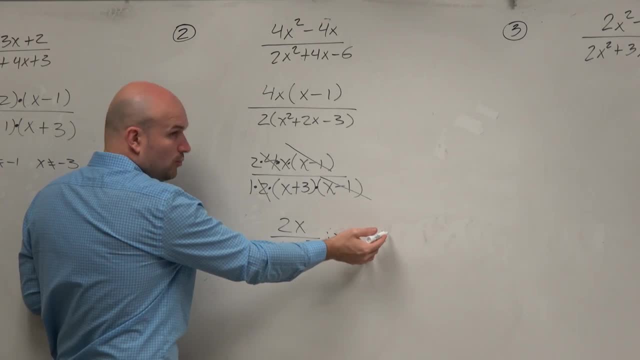 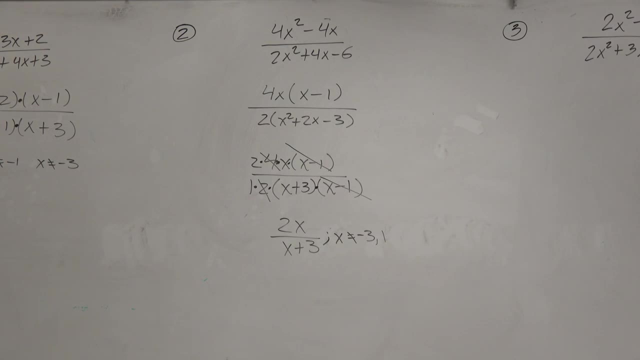 So my 2 undefined values. So my 2 undefined values are: x cannot equal negative 3 or 1, because those would have made that 0. And again, you know it gets to the confusing part of, but it got divided out. Why is it still, you know, not undefined?